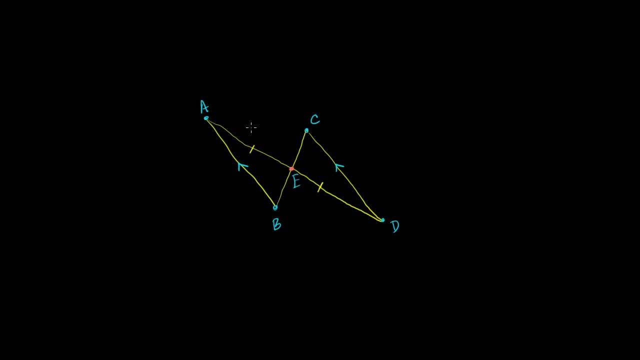 midpoint or is the midpoint of line segment A D? And what I want to think about in this video is: is point E also the midpoint of line segment B C? This is the question right over here. So is E the midpoint of line segment B C? 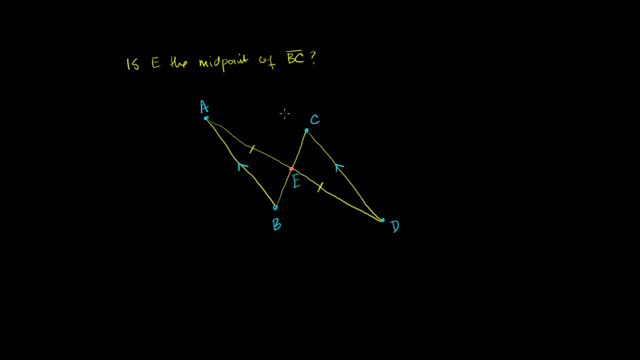 And you can imagine Basically. And you can imagine because this is the most common answer to a lot of the videos we've been seeing lately. maybe it has something to do with congruent triangles. So let's see if we can set up some congruency relationship. 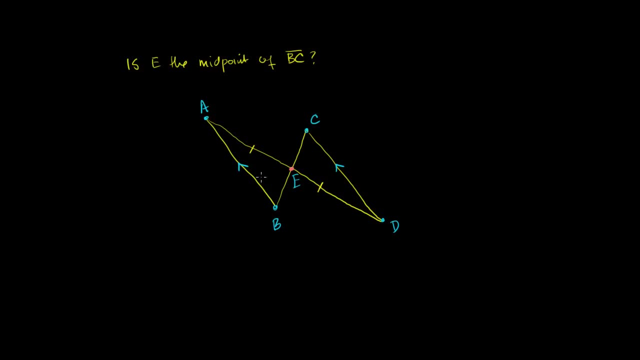 between the two obvious triangles in this diagram. We have this triangle up here on the left and we have this diagram down here. This one kind of looks like it's pointing up, This one looks like it's pointing down. So there's a bunch of things we know about vertical angles. 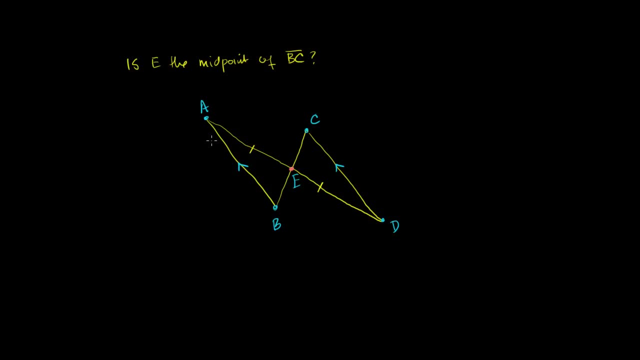 and angles of transversals. The most obvious one is that we have this vertical. We know that angle AEB is going to be congruent, or its measure is going to be equal to the measure of angle CED. So we know that angle AEB is going to be congruent to angle. 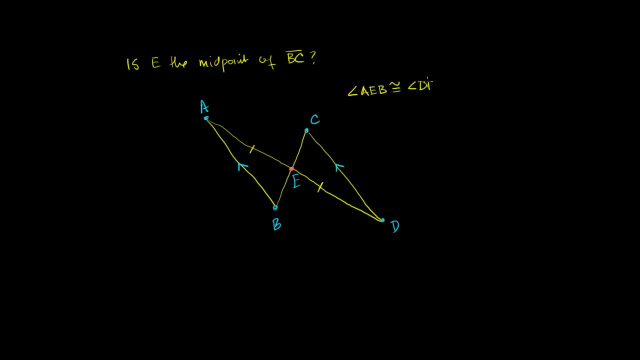 DEC, which really just means they have the exact same measure. And we know that because they are vertical angles, Vertical, they are vertical, they are vertical angles. Now we also know, we know that AB and CD are parallel. So this line right over here, this is a transversal. 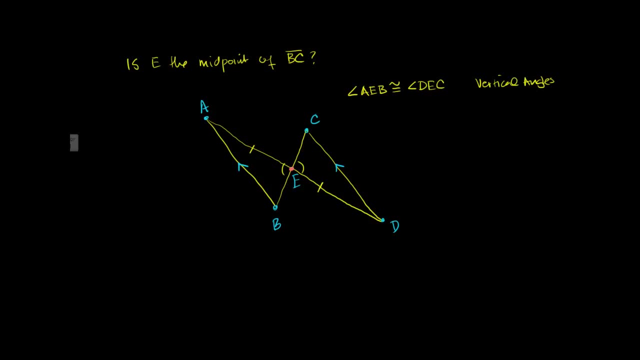 So we know, for example, and there's actually several ways that we can do this problem, but we know that this is a transversal and there's a couple of ways to think about it right over here. So let me just continue the transversal, so we get to see. 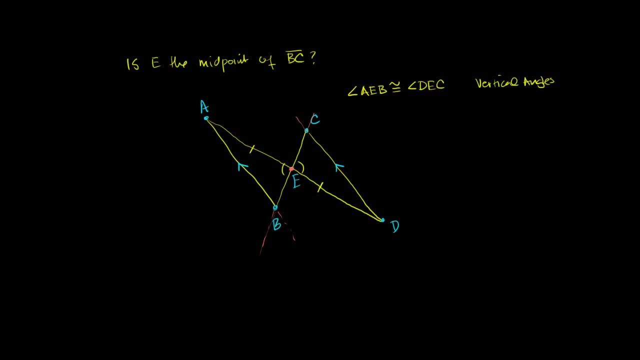 all of the different angles. You could say that this angle, this angle right here, is going to be congruent, or its measure is going to be equal to the angle ABE, So this is its measure right over here. You could say that it is the alternate interior angle to. 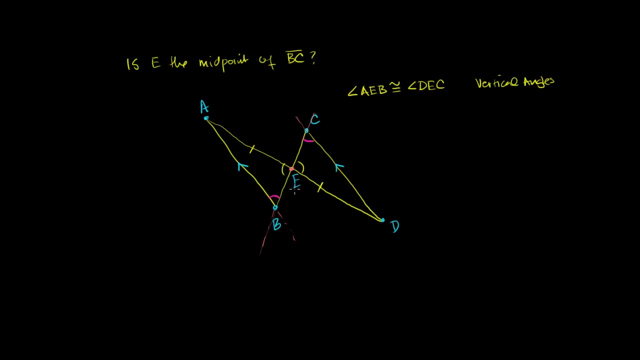 angle ECD to this angle right over there, And if that didn't jump out of you, you would say that the corresponding angle to this one right over here is this angle right up here. If you were to continue this line off a little bit, these: 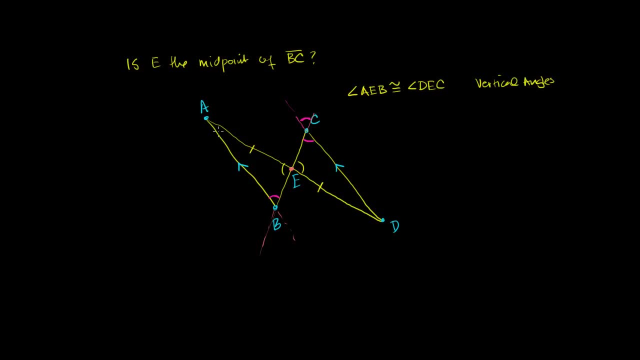 are the corresponding angles, and then this one is vertical, But either way, angle AEB. let me write this down, Sorry. angle ABE- let me be careful. Angle ABE is going to be congruent to angle, so that's. 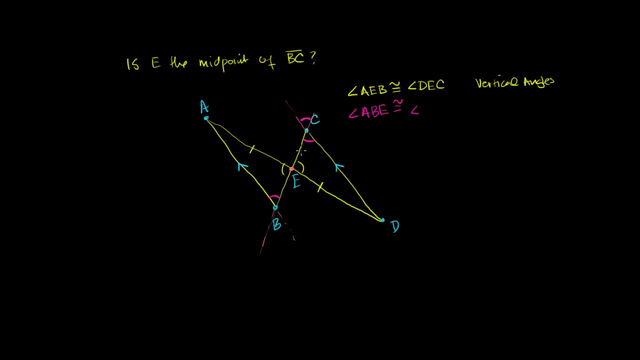 ABE is congruent to angle DCE. It's congruent to angle DCE And we could say: because it's alternate, interior angles Alternate. I'll just write a little code here: So alt interior Angles, And then we have an interesting relationship. 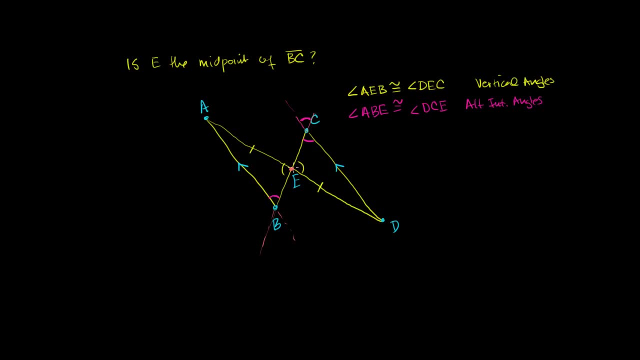 We have an angle congruent to an angle, another angle congruent to an angle and then the next side is congruent to the next side over here. So pink green side, So we can employ AAS angle angle side. 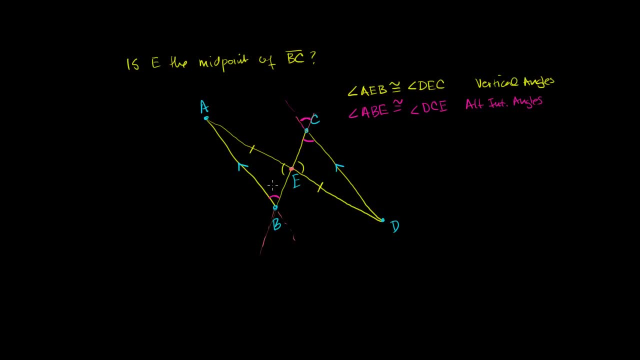 And it's in the right order. So now we know that triangle, we have to make sure that we get the letters right here, that we have the right corresponding vertices. We can say that: triangle, AEB. Actually, let me start with the angle, just to make it. 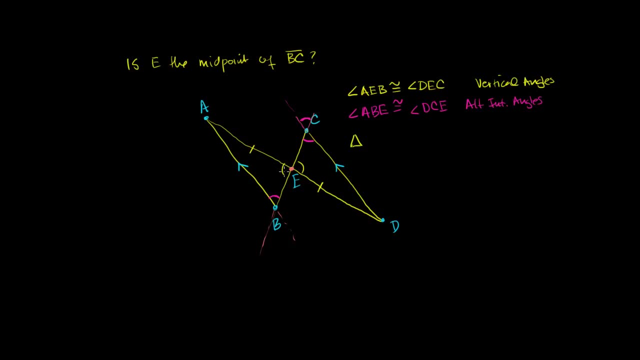 interesting Angle BEA. so we're starting with the magenta angle, going to the green angle and then going to the one that we haven't labeled. So angle BEA we can say is congruent to angle. We start with the magenta vertices. 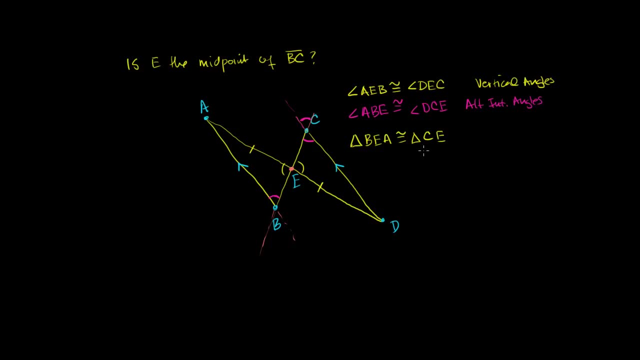 C, go to the center E and then go to the unlabeled one, D, And we know this because of angle, angle side, And they correspond to each other: Magenta green side. Magenta green side. 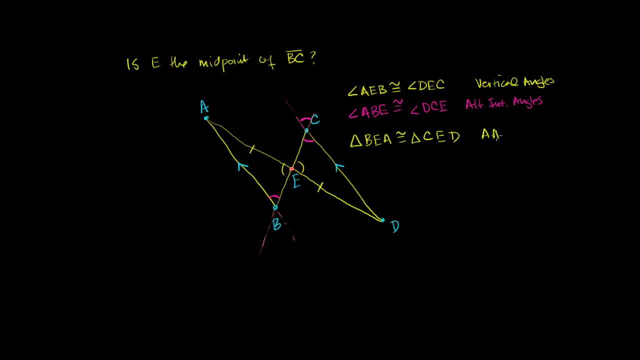 They're all congruent. So this is from AAS, And then if we know that they are congruent, then that means corresponding sides are congruent. So then we know that this side, so we know these two triangles are congruent. 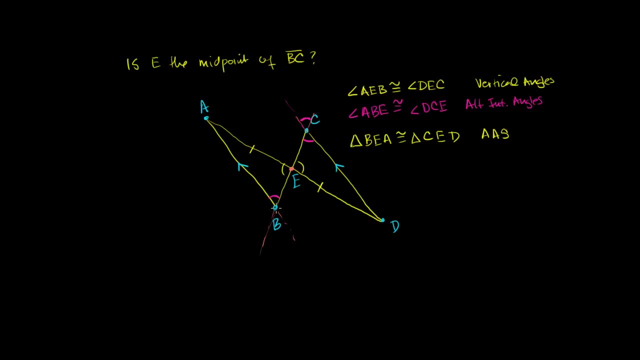 So that means that their corresponding sides are congruent. So then we know that length of BE, the length of that segment BE, is going to be equal, And that's the segment that's between the magenta and the green angles. The corresponding side is side CE, between the magenta and the